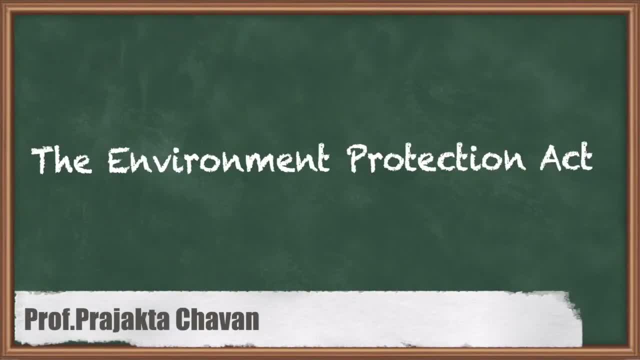 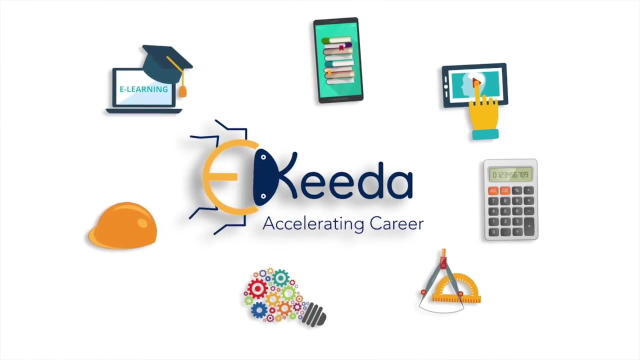 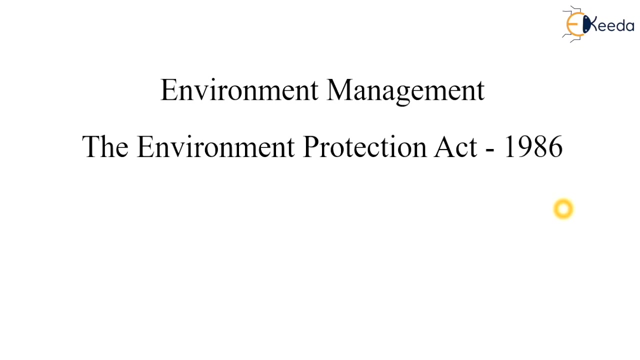 Hello everyone. In this lecture we are going to see the Environmental Protection Act 1986 under the subject of Environmental Management. In this act we are going to see what are the criteria for providing this act and when we are implementing this act. that means, under which criteria we are implementing this act. 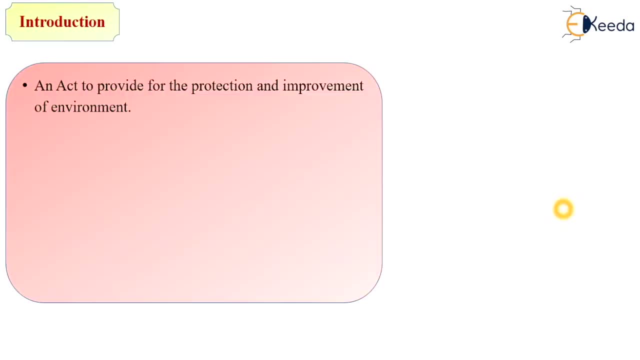 So let's see what is Environmental Protection Act. It is an act to provide for the protection and improvement of environment, Whereas the decision were taken at the United Nations Conference on the Human Environment Act, held at Stockholm in June 1972, in which India participated, to take appropriate step for the protection and improvement of human environment. 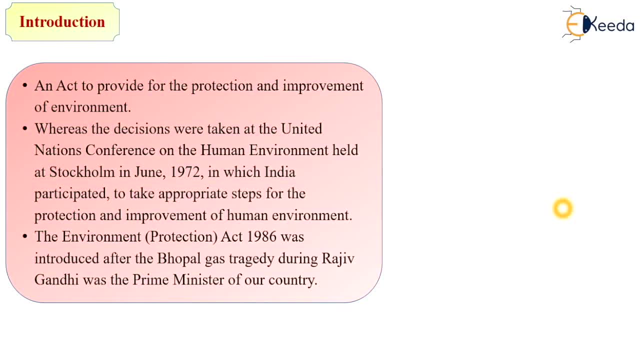 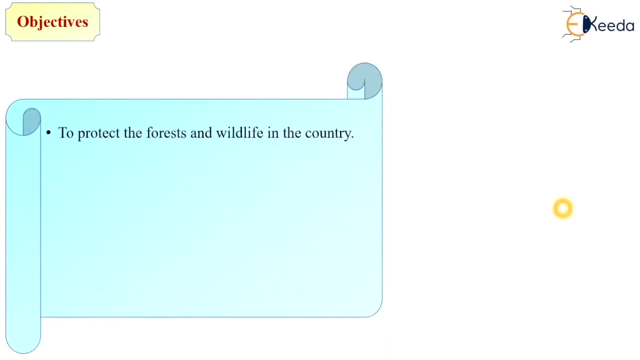 So the Environmental Protection Act 1986 was introduced after the Bhopal gas tragedy. So everybody know that tragedy During Rajiv Gandhi's was the Prime Minister of her country. So the objectives of providing this act is to protect the forest and wildlife in the country. to improve the quality of life by protection of environment. to coordinate the activities of the various regulatory agencies already in existence. 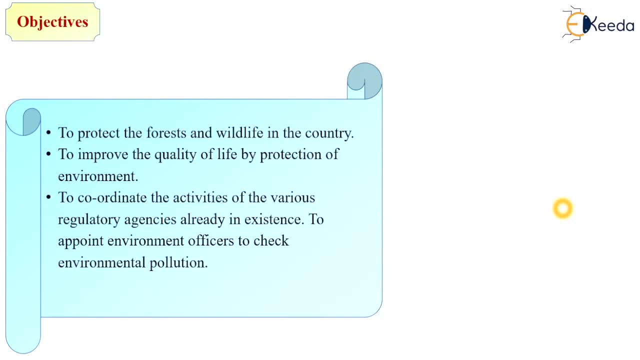 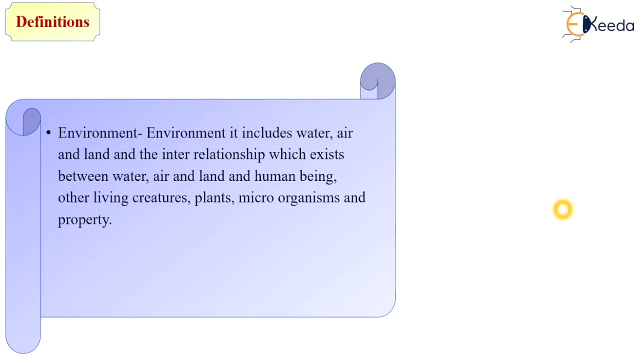 to appoint environment officers to check the environment. So these are some objectives of providing Environmental Protection Act. So there are some basic terms that we should have to understood in when we are following this act. So most important is environment. What is environment? 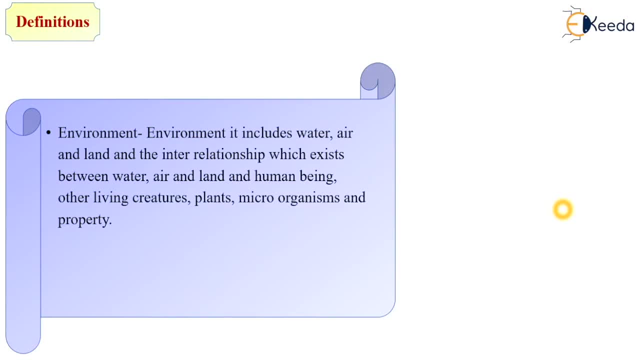 Environment. it include water, air and land And the interrelationship which exist between water, air and land, and human being, Other living creatures, plant microorganisms and property are also the part of environment. What is mean by environment pollutant? 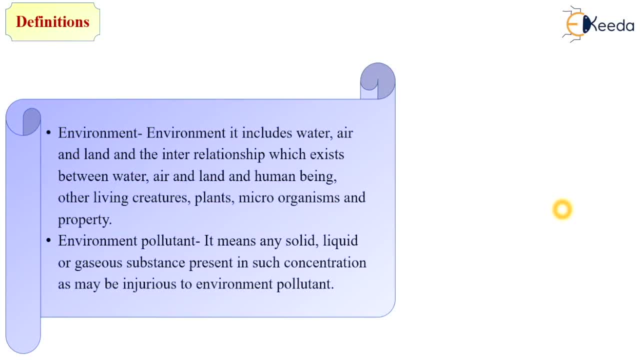 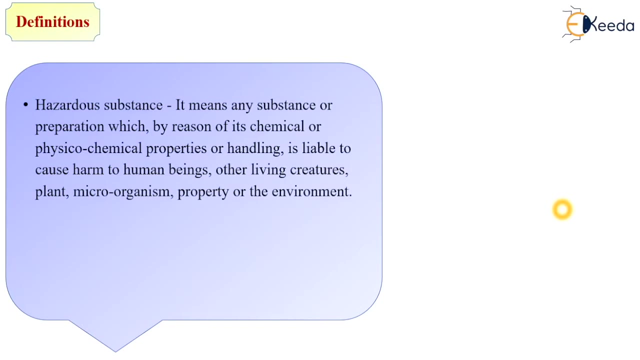 It means any solid, liquid or gaseous substances present in such concentration as may be injurious to environment pollutant. Next is hazardous substances. It means any substance or preparation which, by reason of its chemical or physicochemical properties or handling, is liable to cause harm to you, human being, other living creatures, plant, microorganisms or property or the environment. 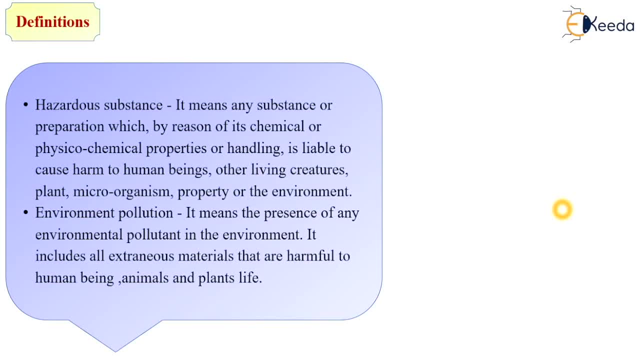 So that substances we are called it as hazardous substances. Next term is Environmental Pollution, Environmental pollution, Environmental pollution: It means the presence of any environmental pollutant in the environment. It include all extraordinary material that are harmful to human being, animal and plant life. 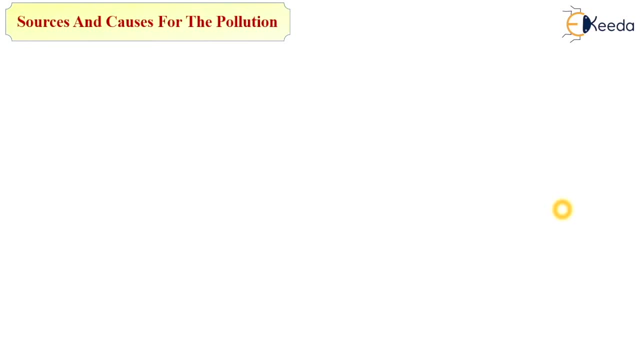 Next is sources and causes for the pollution. What are the sources and causes of environmental pollution? The main cause is combustion. Combustion means burning. Next is pollution, Next is construction activities, Next is mining activities, agricultural activities, chemical plants, coal-fired power plant, oil refineries, petrochemical plant, nuclear waste, large livestock farm like poultry, dairy cows, etc. 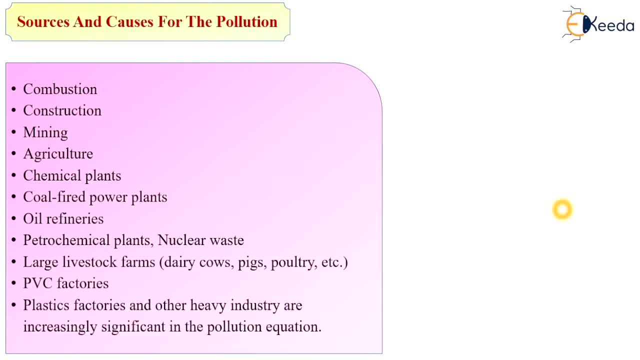 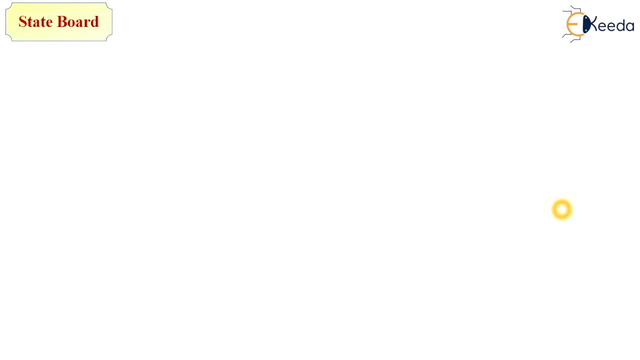 Polyvinyl chloride factories, preparation of PVC pipe factories, plastic factories and other heavy industries are increasingly significant in the environment. They are mostly significant in the pollution equation. So that are the main sources and causes for the environmental pollution. So, as you all of know, because of urbanization and industrialization the pollution and environmental pollution goes on increasing and increasing and we have to reduce this pollution and because of that we are implementing the Environmental Protection Act to protect our environment. 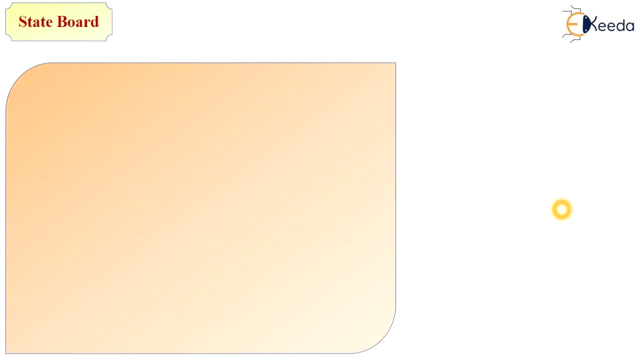 So for that, the state government ruled some policies, ruled some policies. So let's see what are that policy or what are that hierarchy of the state board. The first person in the state board is chairman. Next is the representative of the state government. These are the quantity of that representatives are less than 5.. Next is the. 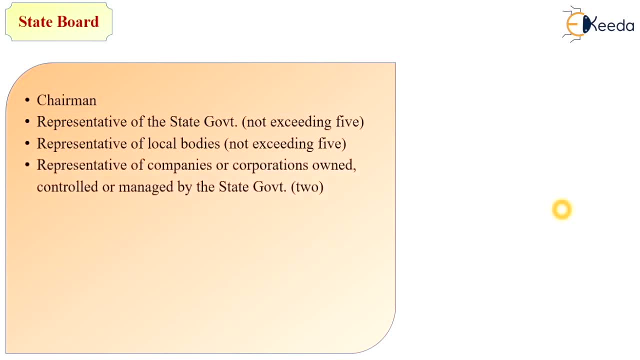 representative of local bodies, not exceeding 5 number. Then the representative of companies or corporations owned, controlled or managed by the state government. There are minimum two quantities. Next is the representative have interest of agriculture, fishery or industry or trade, etc. That member should not exceeding 3 numbers. Next is the member secretary. 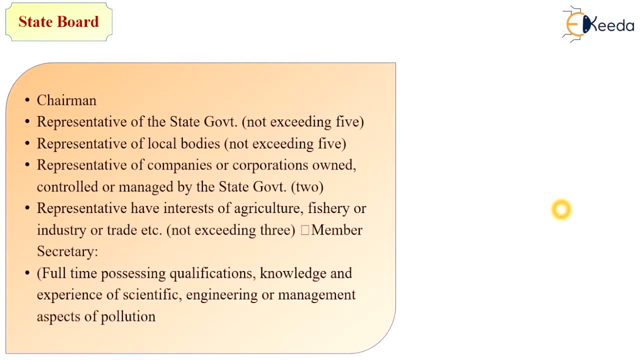 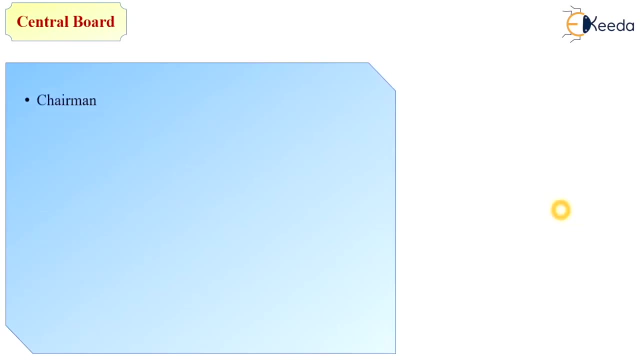 which is full-time, possessing qualification, knowledge and experience of scientific engineering and management aspect of pollution. So this is the hierarchy of state board, Then the central board. Under central board, again, chairman is there. Then the representative of the central government, The quantity of that members are not exceeding 5. Then the representative of state. 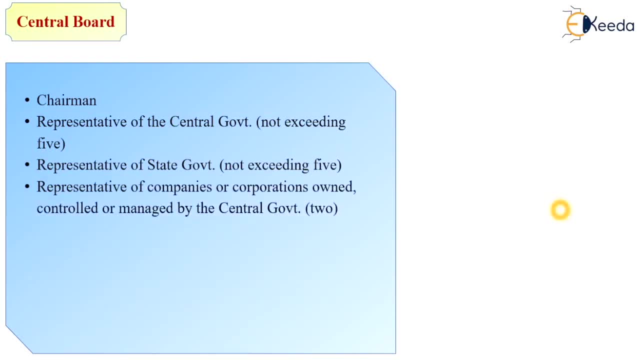 government not exceeding 5.. Then the representative of companies or corporations owned, controlled or managed by the central government. The quantity member of that representatives are 2.. Then the representative of central government should be nahe affeka303151 of adding meaning to tracks codes, So since that member will have the personality to facing a significant 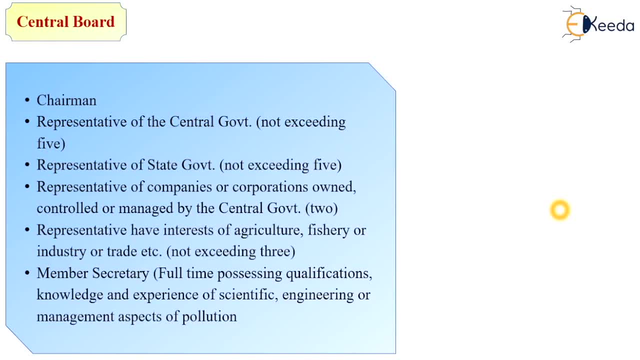 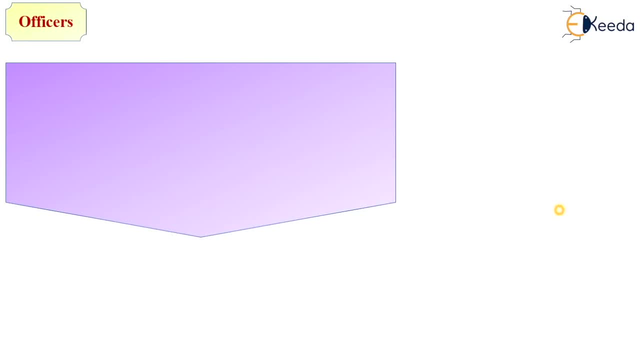 weight of costombality. wszystkie необходien 가자 afer costs are 귀 10 enjoy to pay all the cost of maintenance of the pane name. Belarusian Ten falling down. There are three poorAmericans in one daily basis: Topudi Eye 7.. Then representative have interest of agriculture, fishery. 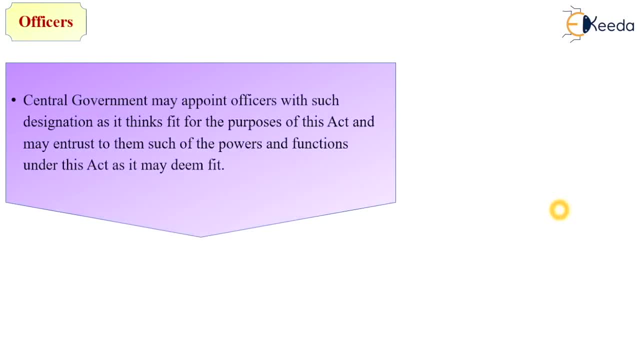 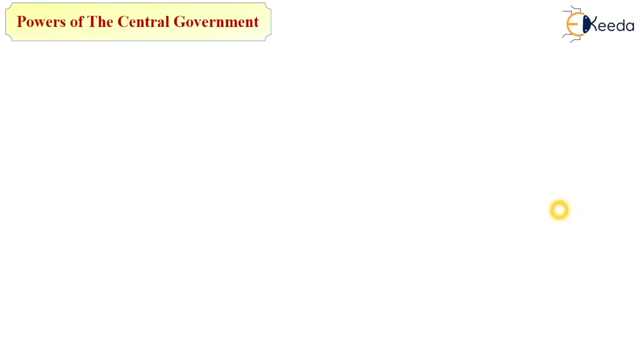 Central government may appoint officers with such designation as it think fit for purpose of this act, and may entrust to them such of the powers and functions under this act as it may deem fit. So what are the powers of central and state government? So let's we see one by one. 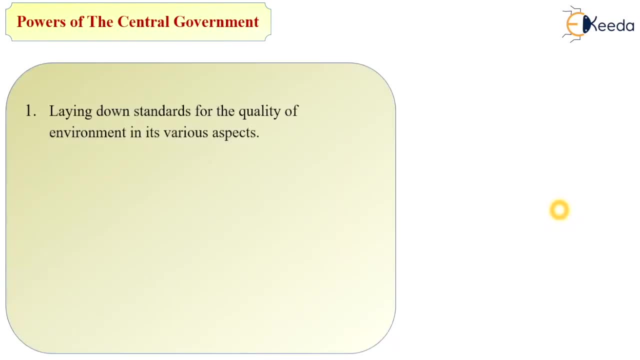 So first is the power of central government. under this Environmental Protection Act, Central government should laying down standards for the quality of environment in its various aspects, Planning and execution of nationwide program for the prevention, control and abatement of environmental pollution. Next, the laying down standards for emissions or discharge of environmental pollutants from various sources. 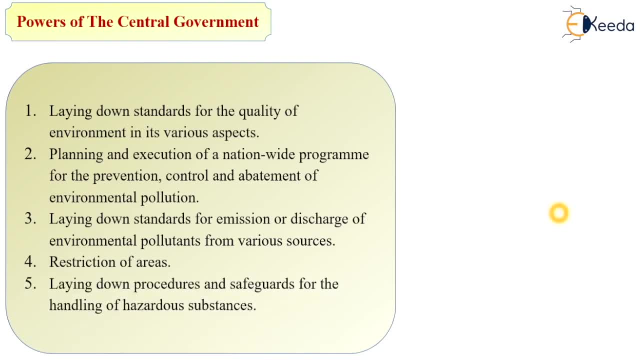 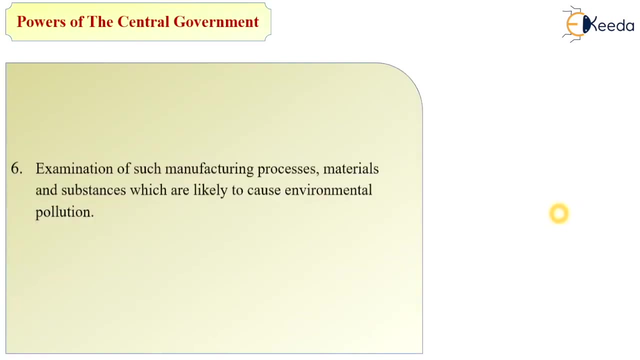 Next, the restrictions of areas and laying down procedure and safeguard for the handling of environmental pollution. Next, the laying down of hazardous substances. So these activities under takes place, taken by the central government. Again, examination of such manufacturing processes, materials and substances which are likely to cause the environmental pollution. 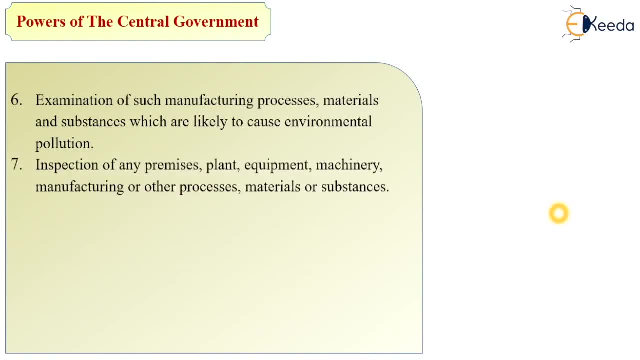 Again, central government take care of these activities. Then the inspection of any premises, plant, equipment, machinery, manufacturing or other processes, Materials or substances. Then establishment or recognition of environmental laboratories and institutes. Then collection and dissemination of information in respect of matter relating to environmental pollution. 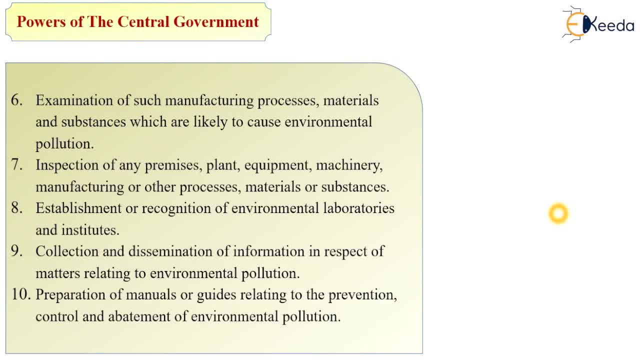 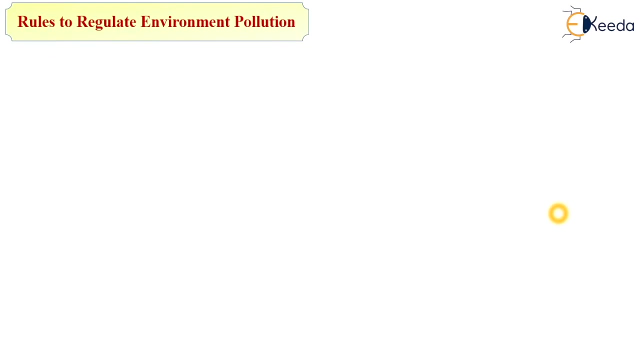 And preparation of manuals or guidelines relating to the prevention, control and abatement of environmental pollution. So these are the power under the central government through that The central government can conducting such activities by the representative of central government. Next is the rules to regulate the environmental pollution. 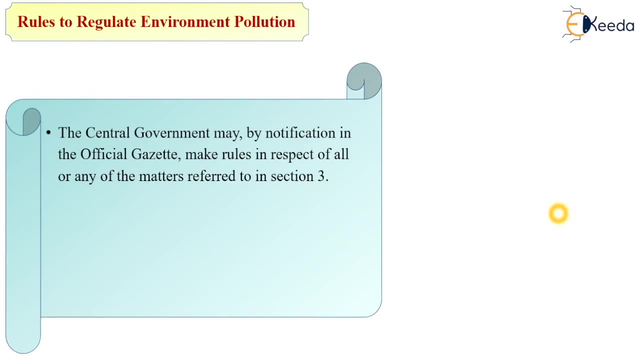 Which rules are involved in this environmental pollution or environmental protection act. The central government may, by notification in the official gazette, make rule in respect of all or any of the matter referred to in section 3.. First, the standards of quality of air, water or soil for various area and purposes should examine. 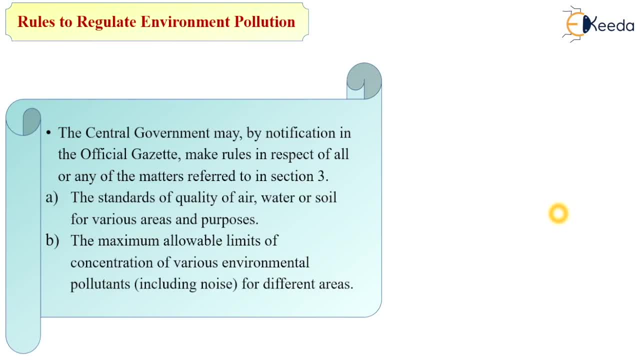 the maximum allowable limit of concentration of various environmental pollutant for different areas. So these are some activities. The central government have control on this activity or they should decide the standards or quality of this. Disha standards, Again, the procedures and safeguard for the handling of hazardous substances. 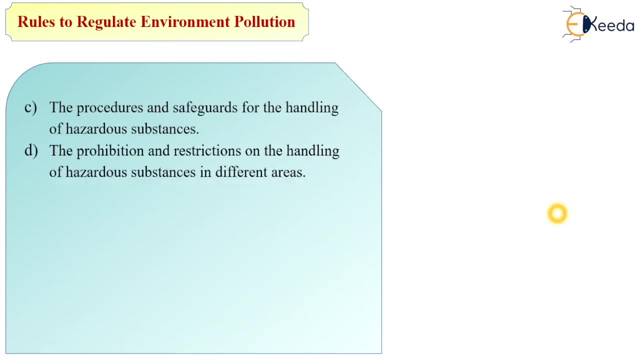 The prohibition and restrictions on the handling of hazardous substances in different area. For example, the central government has rights to rule on the hazardous waste management or to set the limits on them or to take the action on them. Then the prohibition and restrictions on the location of industries and carrying on process and operations areas. 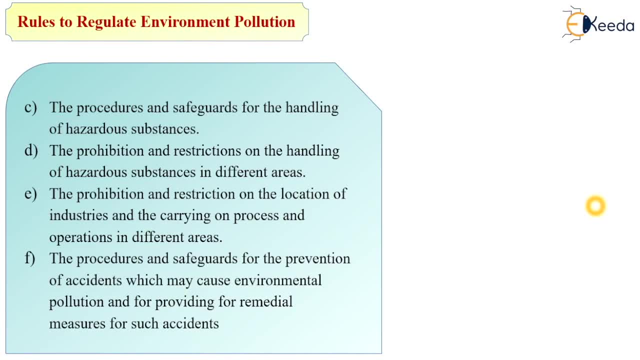 The next is the procedure and safeguard for the handling of hazardous substances, Then the prohibition and restrictions on the handling of hazardous substances in different area. That means the central government has rights to prohibit the particular area which is impact, which is affect the environment and which cause the environment because of exceeding the limit of hazardous substances. 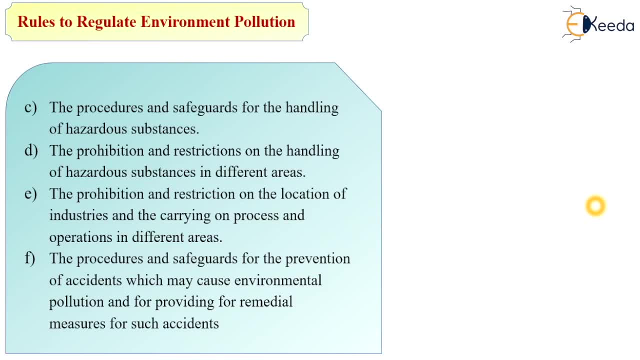 So central government has right to set the limit or prohibition of any area which are increasing the environmental pollution. Then the prohibition and restrictions on the location of industries and carrying on process and operations in different areas. The procedure and safeguard for the prevention of accident which may cause the environmental pollution and for providing for remedial measures for such a accident. 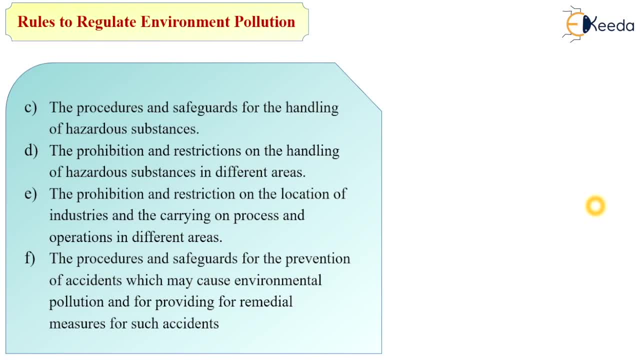 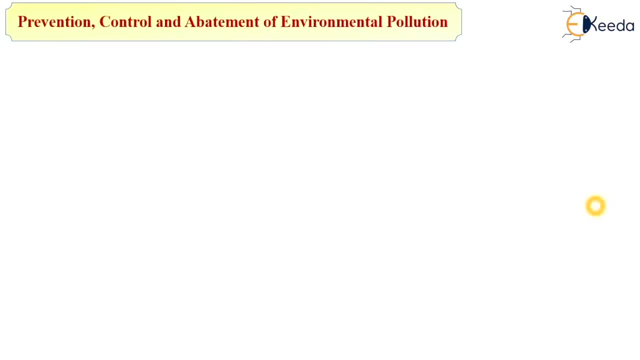 So central government has each and every right, which is reducing the part of environmental pollution. The next is prevention, control and abatement of environmental pollution. So how we can contribute to reducing the environmental pollution, The person carrying on industry operations, etc. not to allow emissions or discharge of environmental pollutants in excess of the standards. 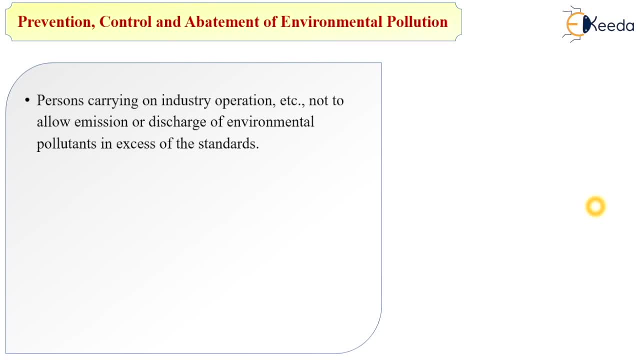 So for that the central government has set some permissible limits for discharge standards. That means the industries will not discharge directly its effluent without any treatment. So nowadays the industries has it has a compulsory to treat the waste water generated from each and every industries. 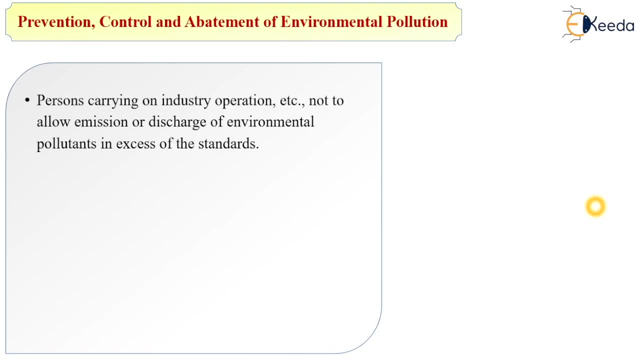 And when its standards are matched with the permissible limit or discharge standards, then, and only then, it will discharge into the water bodies, Unless otherwise the central government has Take some serious actions on that. Sometimes the industry, many of industries, may get banned because of that they are not matching the discharge standards. 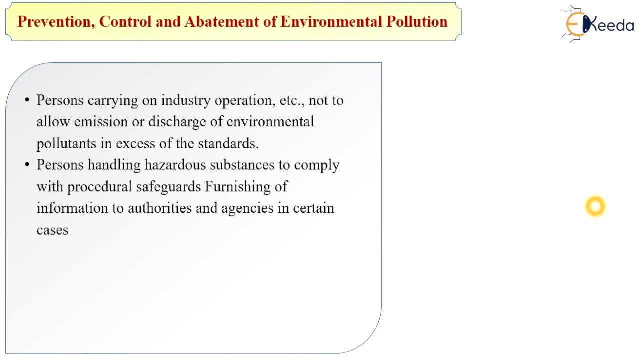 Then the persons handling hazardous substances should to comply with procedural safeguard, furnishing of information to authorities and agencies in certain cases. Then the power of entry and inspection, Power to take sample and procedure to be followed in connection therewith, And environmental laboratories has set by central government and testing is done by in this laboratories. 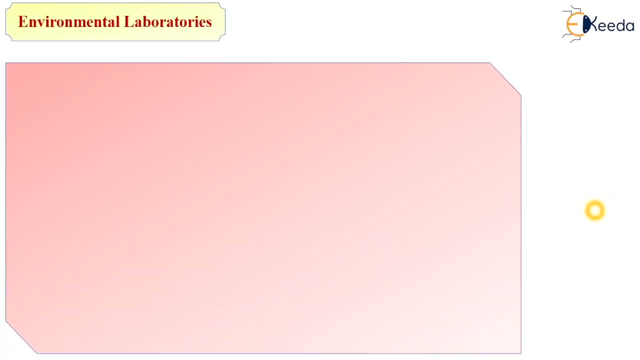 Next the environmental laboratories and it will be the. it must be the part of environmental protection act. So central government has some: the centrally environmental laboratories: Central laboratory, Maharashtra, pollution control board, CID, CO Bhavan, 5th floor, South wing, Belapur. 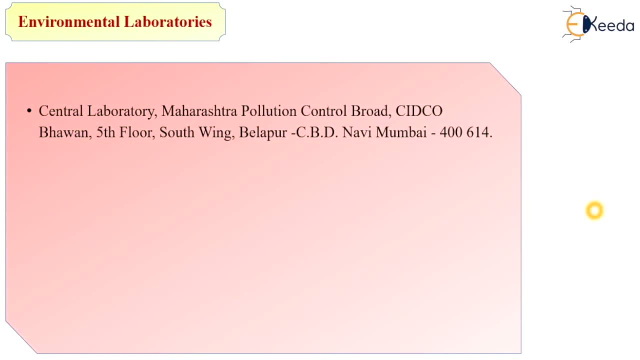 Established in this area, that is, CBD Ravi Mumbai, Then the central laboratory Maharashtra pollution central board Army and Navy building ground floor, 148MG road, Fort Mumbai. The environmental survey laboratory is established at the POTAP district, Thane. 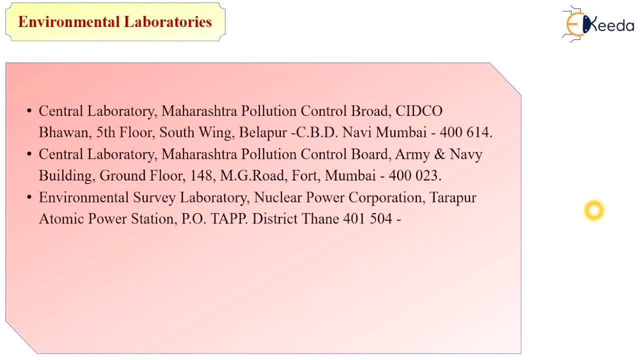 Which related to the nuclear power corporation: Tarapur atomic power station. Next the environmental survey laboratory, the health physics division, Bhabha atomic research centre, Trombe, Mumbai And the chemical laboratory, Indian bureau of mines pore dressing divisions. new secretarian building, civil lines, Nagpur. 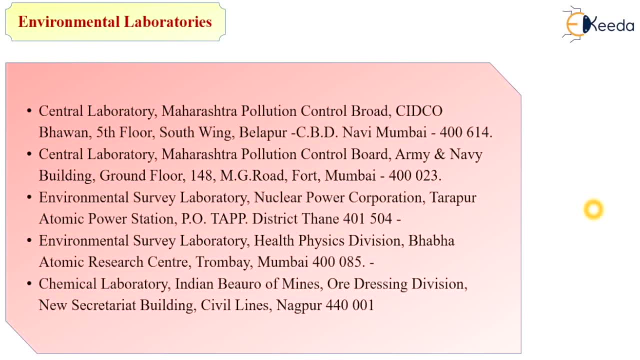 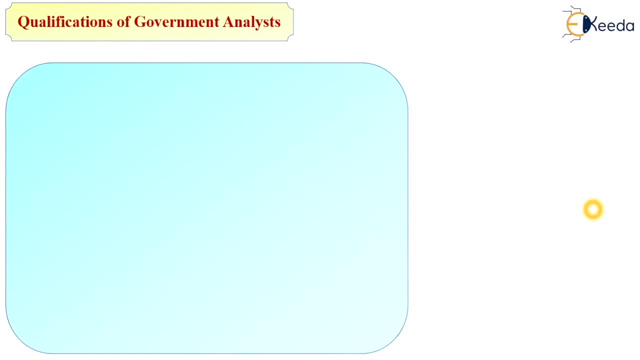 So these are the centrally located laboratories we are established under this environmental protection act all over the India. The next is qualification of Government analysis Graduate in science: the participant or person which will graduate in science from a recognized university, with 5 years experience in the laboratory engaged in environmental investigations, testing or analysis. 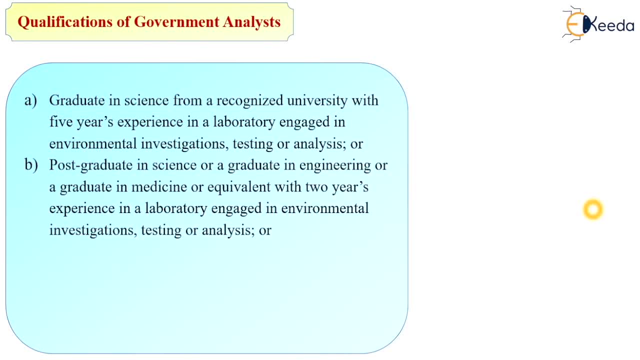 Next post graduating science or graduate in engineering on the graduate in medicine or equivalent, with 2 years experience in the laboratory engaged in environmental investigations, testing or analysis. Or The post graduate in environmental science from a recognized university with 2 years experience in laboratory engaged in environmental investigation, testing and analysis. 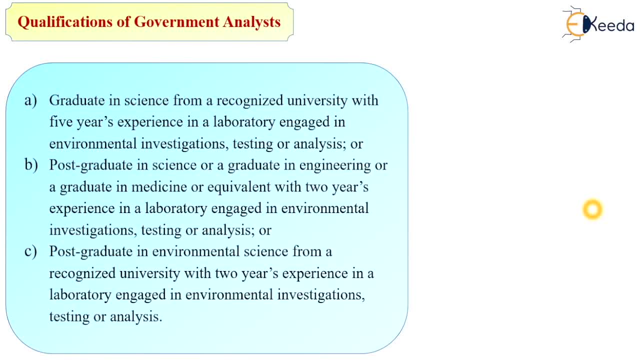 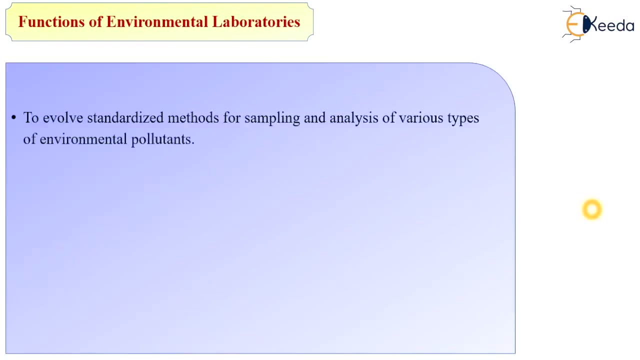 So if any of one of these criteria is matched, then that person will be the part of that testing or environmental laboratories which are centrally established. Then what are the functions of environmental laboratories? To involve standardized method for sampling and analysis of various types of environmental pollutants. 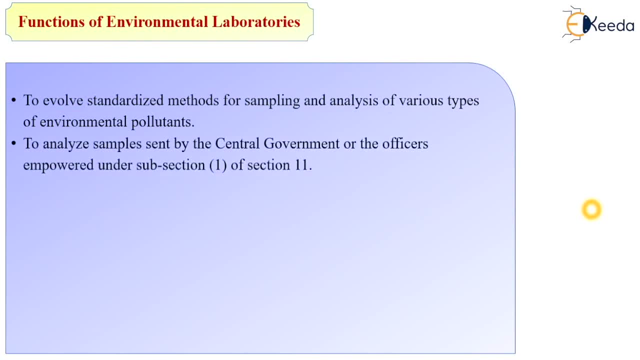 To analyze samples sent by the central government or the officer empowered under the subsection 1 of section 11.. To carry out such investigations as may be directed by the central government. to lay down standards for the quality of environment And discharge of environmental pollutants. to monitor and enforce the standards laid down. 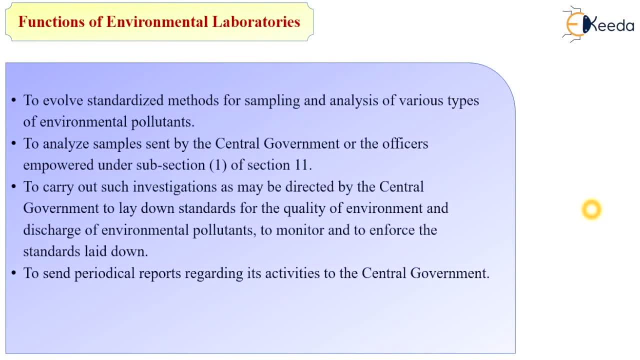 Next, to send the periodic report regarding its activities to the central government and to carry out such other functions as may be interested to it by the central government from time to time. So these are the functions of environmental laboratories which has sent by the central government. 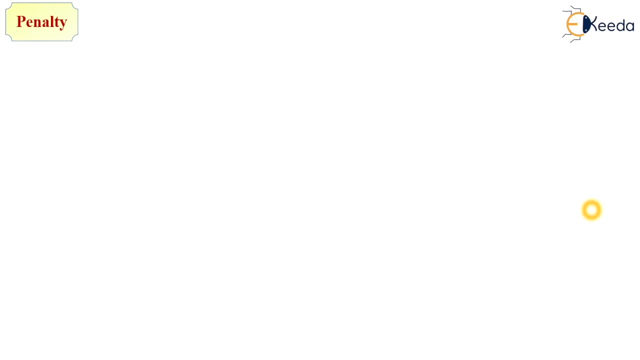 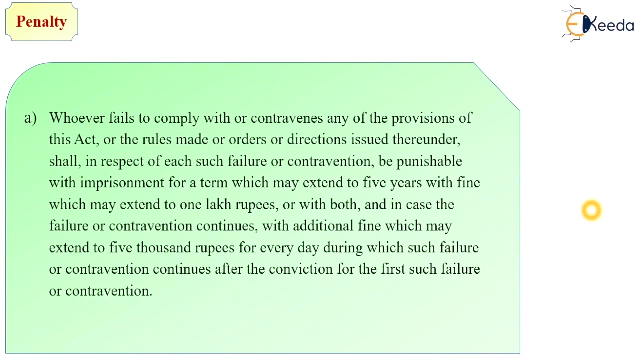 Next is: what are the penalties should apply by the central government when any person or any industry or any organization which are not following this act, environmental protection act. So what are the penalties? First is whoever failed to comply with the contravence, any of the provision of this act or the rules made or orders or direction issued there under. 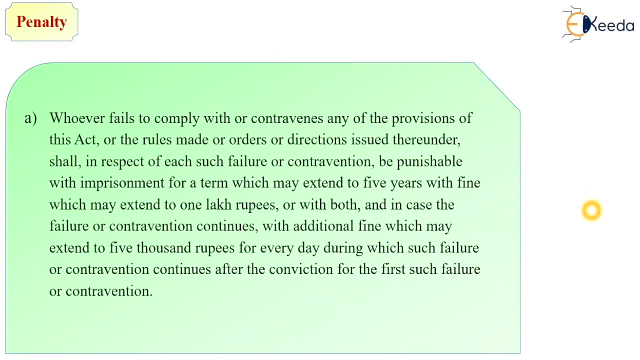 There under shall, in respect of each such failure or contravention, be punishable with imprisonment for a term which may extend to 5 years, with fine which may extend to 1 lakh rupees, or with both, and, in case the failure or contravention continue, additional fine which may extend to 5000 rupees for every day during which such failure or contravention continues. 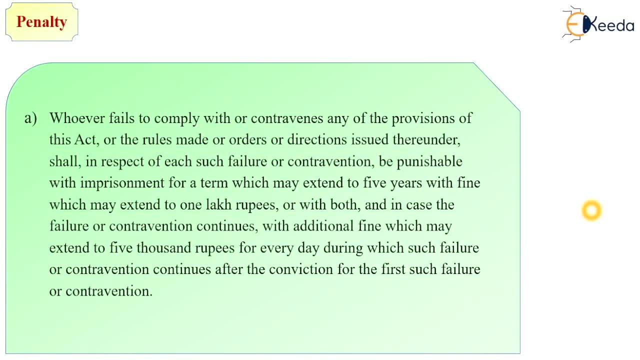 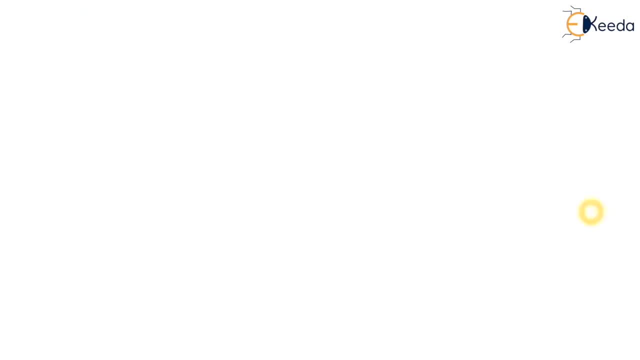 After the conviction for the first such failure or contravention, And if the failure or contravention referred to in subsection Subsection continues beyond a period of 1 year after the date of conviction, the offender shall be punishable with imprisonment for a term which may extend to 7 years. 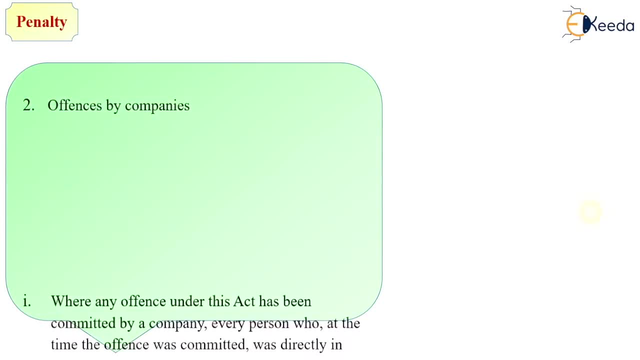 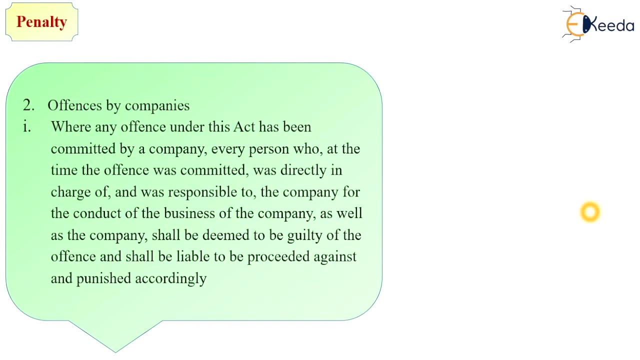 Next punishment is offence by companies. if offence has done by companies, where any offence under this act has been committed by the company, every person who, at the time the offence was committed, was directly in charge of or the part of that offence and was responsible to the company for the conduct, for the business of company as well as the company, shall be deemed to be guilty of the offence. 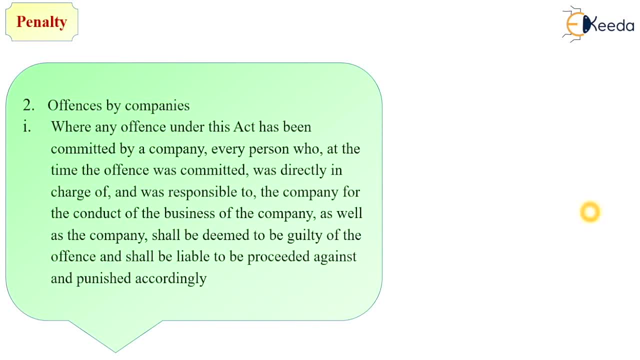 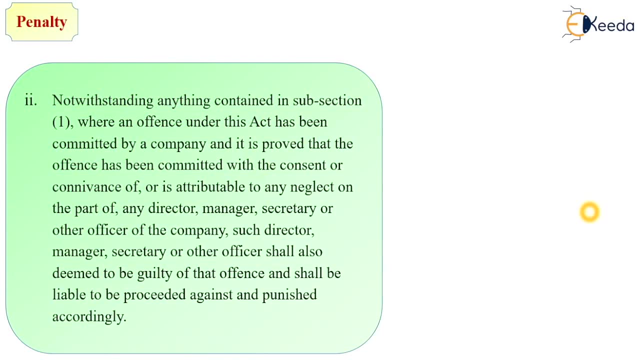 This offence shall be liable to the proceedings against and punished accordingly, Not with standing anything continued its subsection one where an offense under this act has been committed by the company and it is provided that the offense has been committed with the consent or convenience of, or is attributed to any neglected on a. 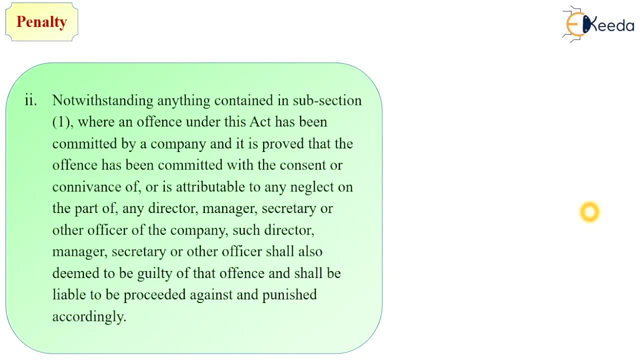 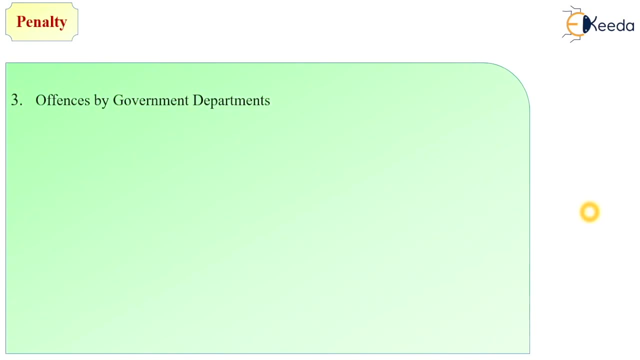 part of any director, manager, secretary or other officers of the company or other officer shall also deem to be guilty of the offense and shall be liable to the proceeded against the punished accordingly. Next offense is by government department, So this is the kind of serious offense. 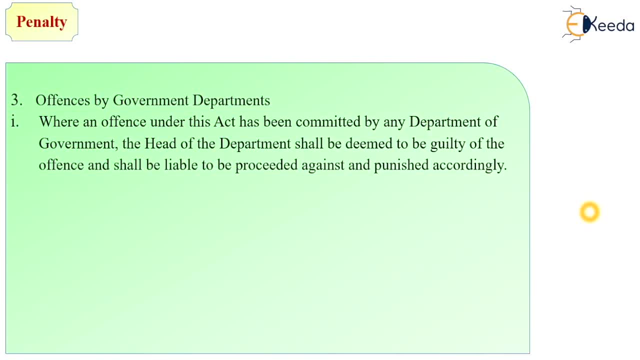 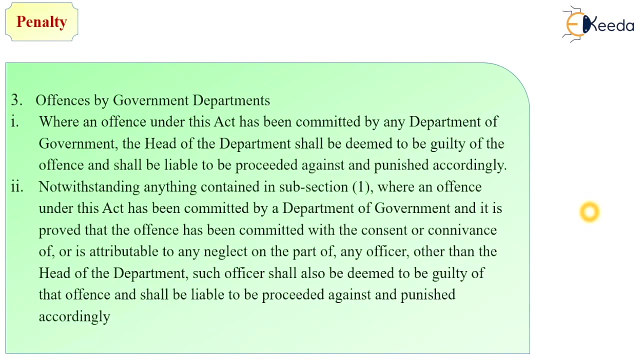 Where an offense under this act has been committed by any department of government, the head of department shall be deemed to be guilty of the offense and shall be liable to be proceeded against and punished accordingly, Notwithstanding anything contained in subsection 1, where an offense under this act has been. 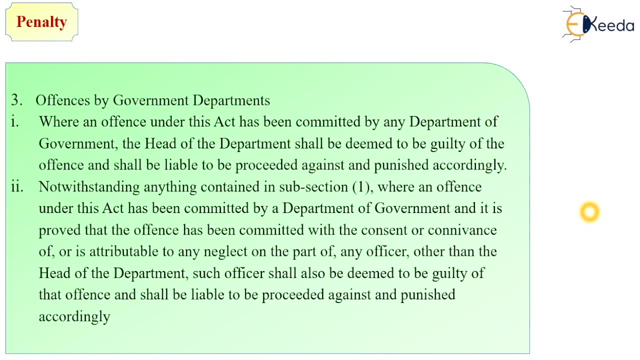 committed by the department of government, and it is provided that the offense has been committed with the consent or convenience of, or is attributable to, any neglect on the part of any officer other than the head of department, such officer shall also be deemed to guilty of that offense and shall be liable to be proceeded against and punished. 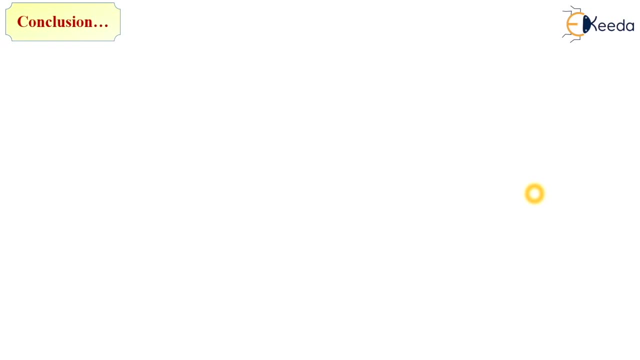 So, by summarizing this act, that is, Environmental Protection Act, we have seen what is the power of central and state government, what are the criteria which are set under this Environmental Protection Act and when we are implementing this act, and which organization and industries which are the part of this Environmental Protection Act.